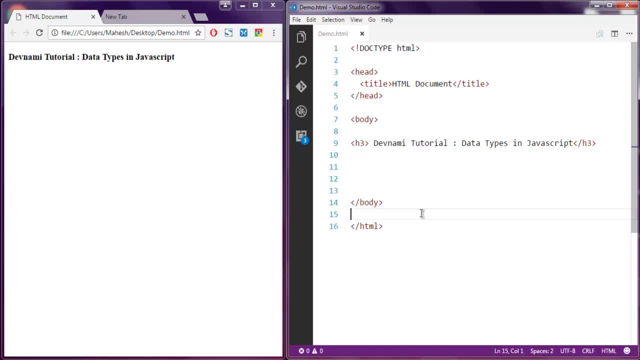 hi there. so in this video, I'm going to talk about data types in JavaScript. so the first thing I want you to do is create an HTML page and add some sample text in it. also, make sure to open that HTML page in a browser. okay, so I'm doing. 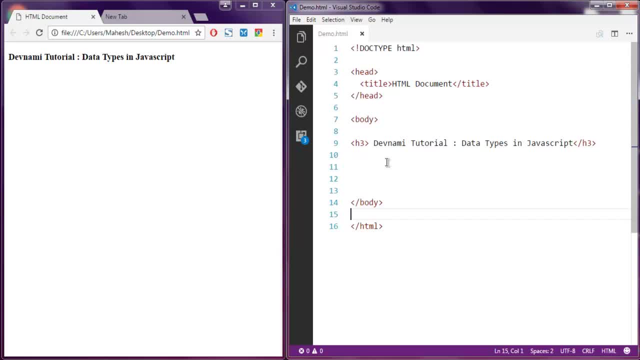 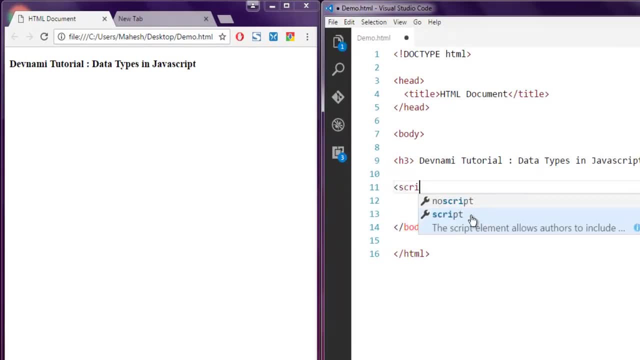 these two windows side-by-side so that you can view it clearly. okay, now, inside your HTML body tag, I want you to add a script tag. okay, make sure to start and close the tag properly, and the first thing I want you to do is initialize a variable. let's say we use a var keyword, then X. okay, right now, as you can see, X. 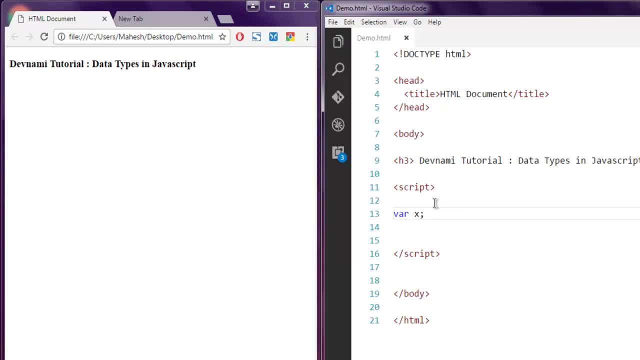 has no value assigned to it, be it string, number, etc. so JavaScript will treat that as undefined variable. so we can use document dot, write and print out value of X and on screen you can see it shows undefined. now what if you give it value? let's say 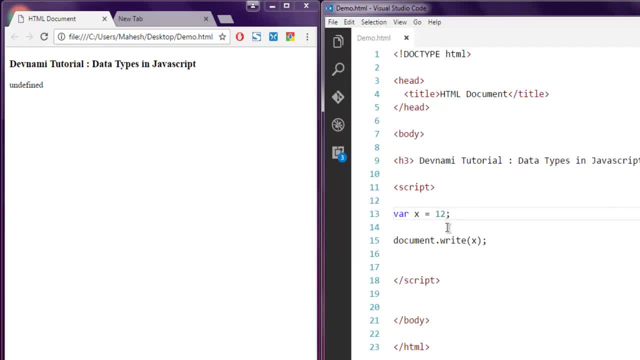 12. okay, now it will hold integer value of 12. it will point that out. that's 12. okay, now what if you give it, let's say, string value, which is, let's say, my channel name, Dev Nami, and I'm going to refresh the page to see if it holds the integer value or string, and 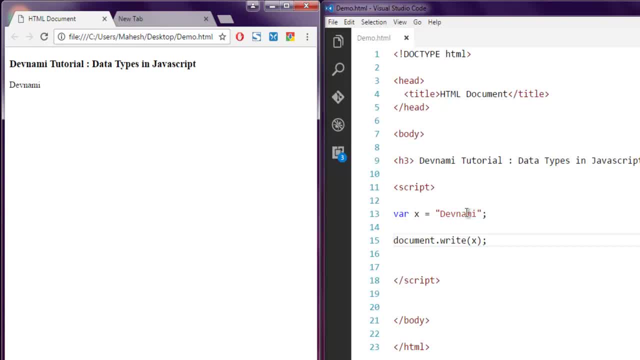 now it will be replaced with string value. now, okay, so you can add a number, string, and also one more type of datatype, which is boolean, which will either hold true or false. so right now, I want to make this variable as true and it will return as true. if it is set to false, to return as false. so you can see.